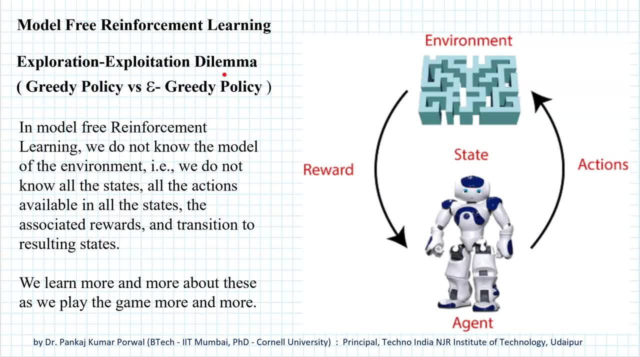 In this session I am going to explain Exploration, Exploitation, Dilemma and Greedy Policy and Absalon. Greedy Policy for Model-Free Reinforcement Learning. In Model-Free Reinforcement Learning we do not know the model of the environment That. 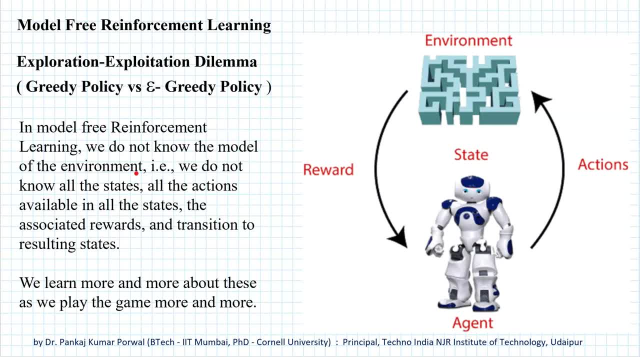 is we do not know all the states in the environment, all the actions available in all the states and the associated rewards and resulting states for taking particular actions in particular states, And we learn about these things by interact with the environment, That is, we 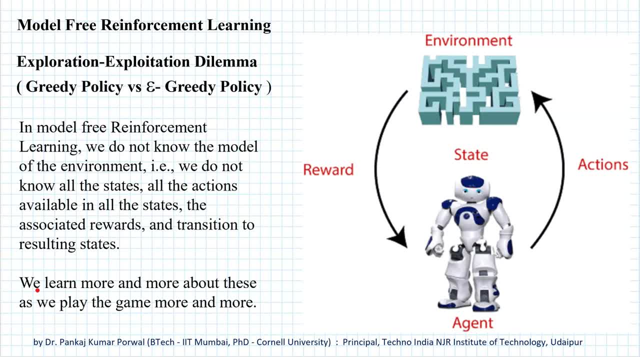 learn about all these things by actually playing the game. And as we play the game more and more, we learn more and more about these things. So, at any given point of time, our knowledge about these things, our knowledge about these things, our knowledge about these things. 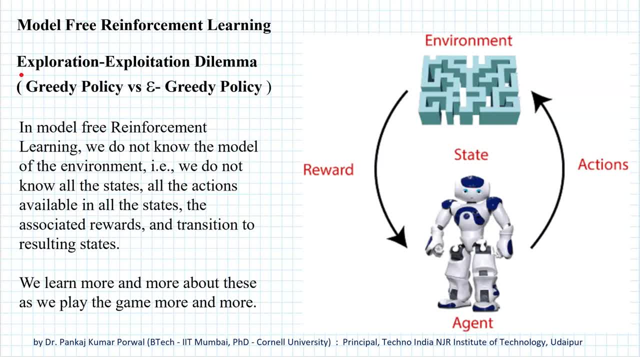 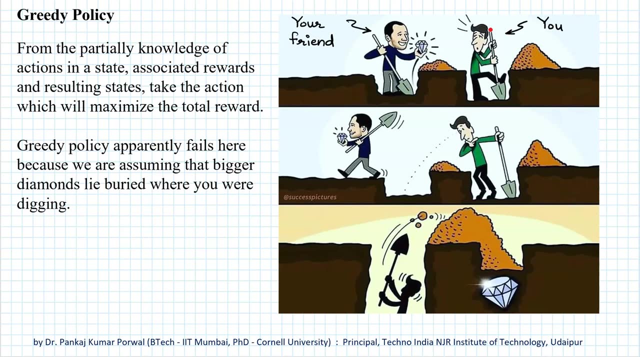 and our knowledge about these things, we are able to learn about these things in the future. states, actions, rewards and resulting states is partial and that's where the exploration, exploitation dilemma comes in. so let us understand that using an example. so let's say you and 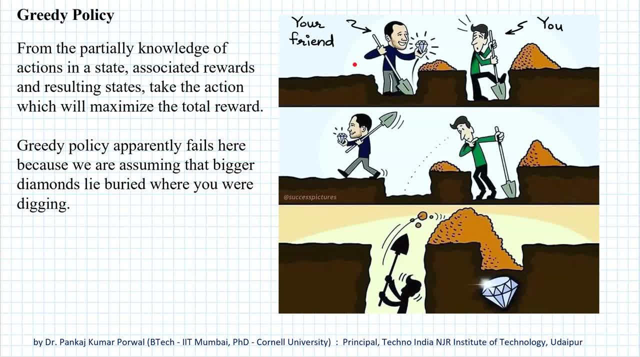 your friend are digging for diamonds and after digging for some time, your friend has found a diamond. now you start thinking whether you should continue digging where you were digging or you jump over to the place where your friend was digging and start digging there. now, if you decide to jump over to the place where your friend was digging, then your 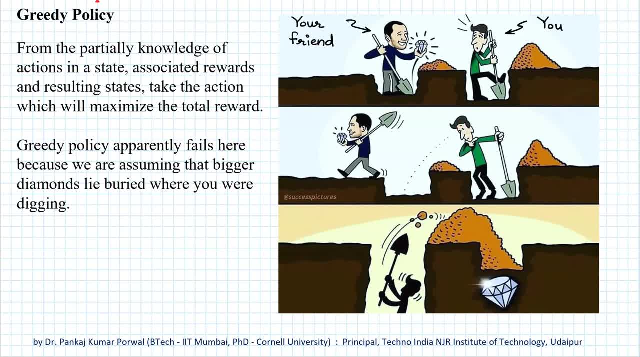 action will be termed as greedy action and the policy that will dictate that action will be greedy policy. Now, in this situation, Our greedy policy apparently fails because we are assuming that bigger diamond lies buried where you were digging initially, but when our friend found a diamond, we only know that. 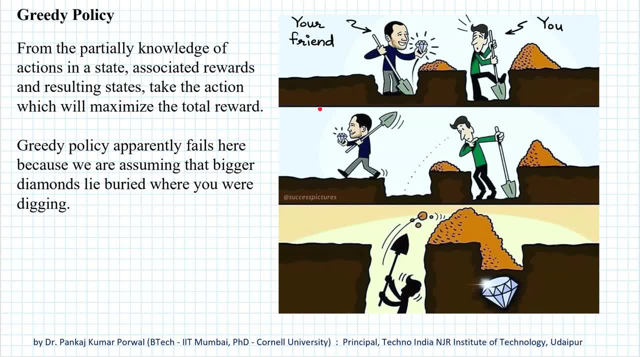 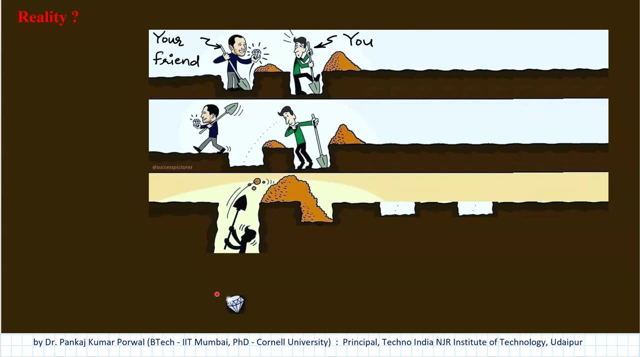 there was a diamond up to this depth at this place, and we do not know exactly what lies under the ground below this level. in reality, the diamond may be where you were digging, or there may be a diamond where your friend was digging, or we may have situation where 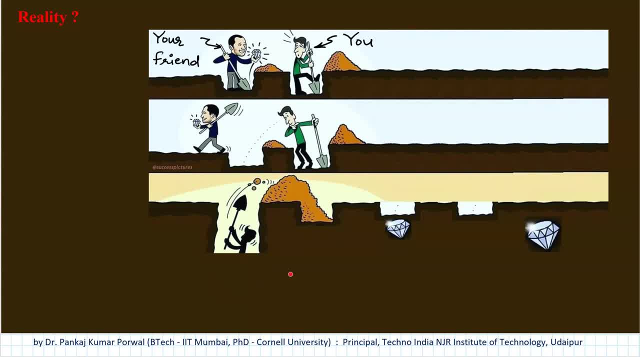 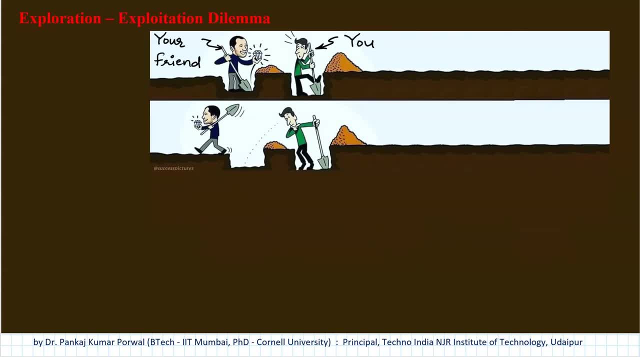 there is no diamond where your friend was digging. there is no diamond where you were digging and the diamonds may be totally at different place. So with this partial knowledge about future states and future rewards, our reinforcement learning agent is in dilemma that whether he should exploit the partial knowledge and 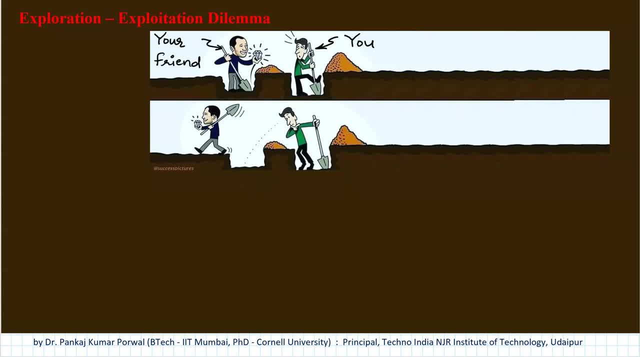 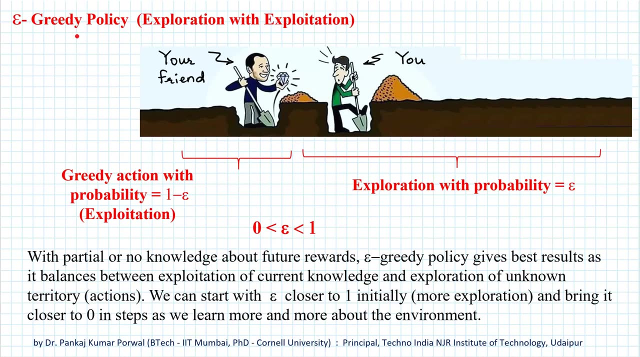 receive Some rewards, or he should explore the unknown actions which may possibly result in much larger rewards. and that's where the concept of epsilon greedy policy comes in, that, with partial knowledge about rewards that we will receive for our actions, we balance between exploitation and exploration. so in our example, when the digging has taken, 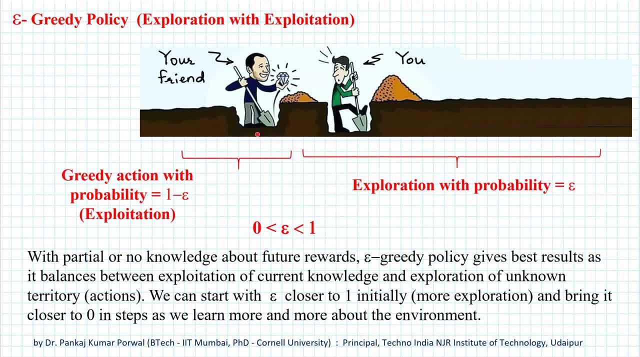 place up to this level. we know that there was a diamond here, so we choose to dig here with probability 1 minus epsilon. that is, we take greedy action or we exploit our knowledge that a diamond was found here and we explore with probability epsilon. that is till now. 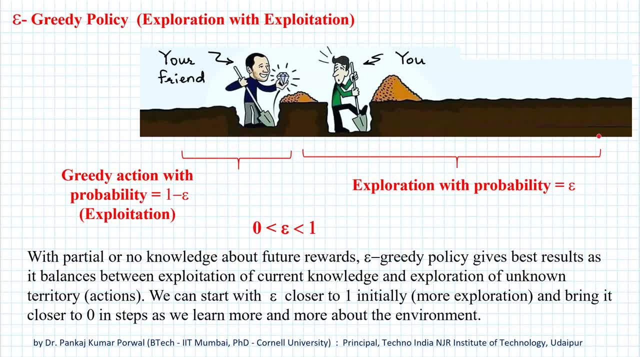 no diamond has been found in these areas, but still we explore these areas with probability epsilon- and here epsilon is a positive real number which lies between 0 and 1, so with partial or no knowledge about future rewards, epsilon- greedy policy gives best results as it balances between exploitation of current knowledge and exploration of unknown territory. 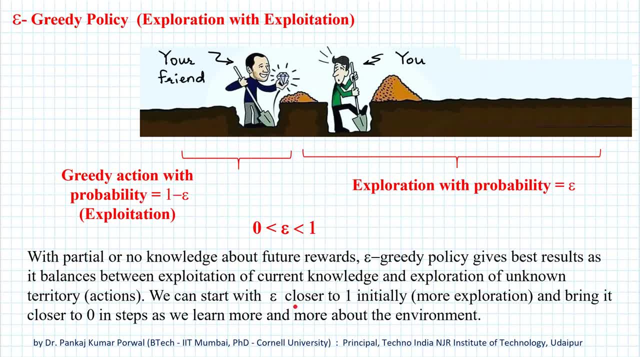 or actions. so we start with epsilon closer to 1 initially, that is, we mostly explore the action when we don't know much about the future rewards that we will receive for our actions, and bring it closer to 0 in steps as we learn more and more about the environment. so as 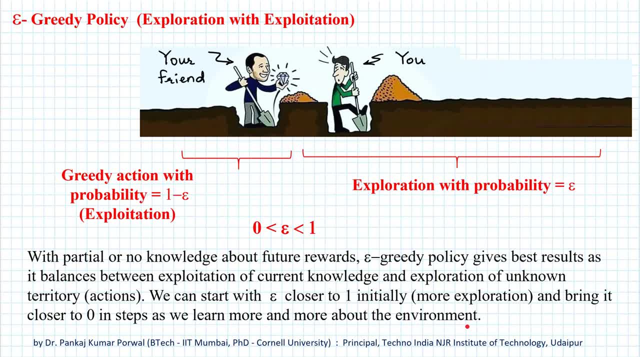 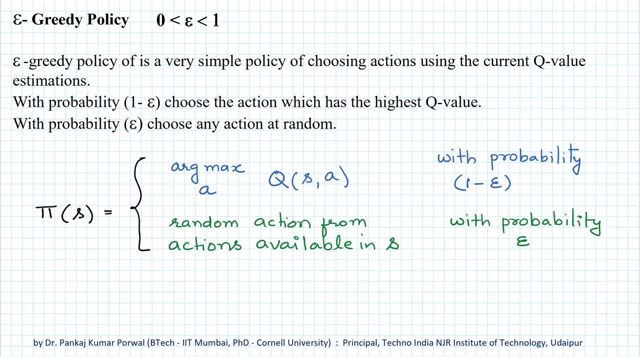 we learn more and more about the environment, we explore less and less and exploit more and more. so mathematically, epsilon, greedy policy, can be written as: with probability 1 minus epsilon, we choose the action a that maximizes the reward and we explore the reward. with probability 1 minus epsilon, that is our action value or Q value in a given state.